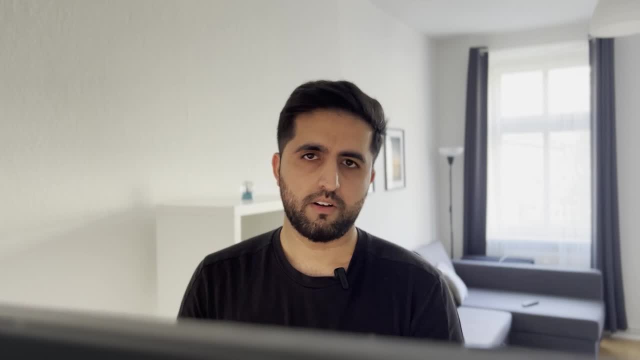 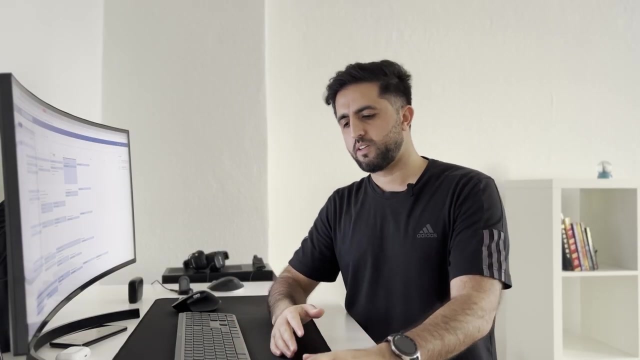 So I thought maybe I should make a video about how I got into QA and maybe I'll be able to give some tips and advice on how you can start your career as well. So let's get started. So, before we get started, I want to explain to you what quality assurance is and what a quality. 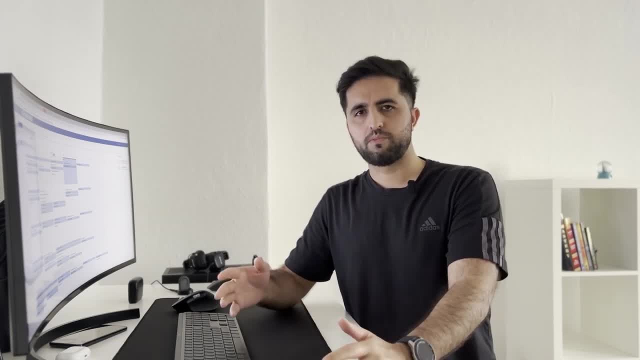 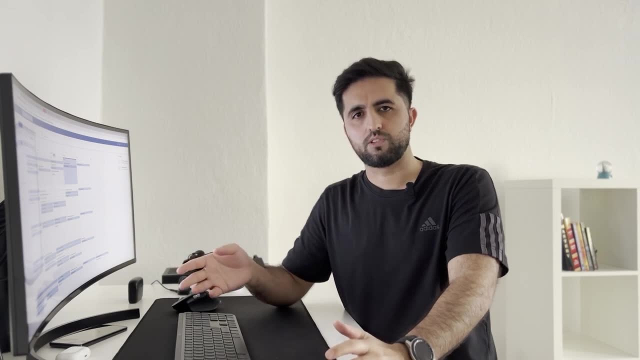 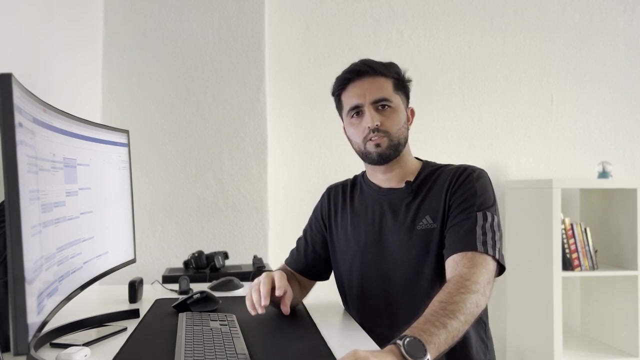 assurance engineer basically does When developing software. the job of a QA engineer is to identify issues or problems or bugs that may arise in future and catch them early on and get them fixed by the developers. Because if these bugs or issues make their way into the production environment or 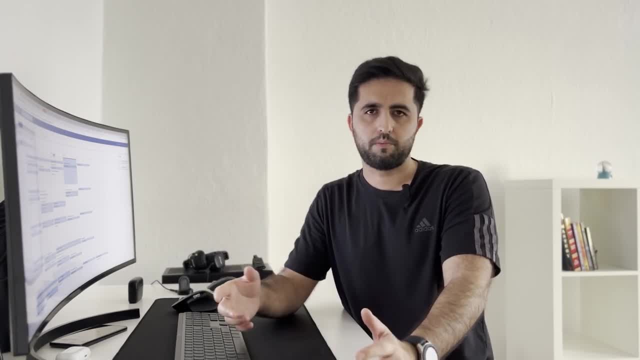 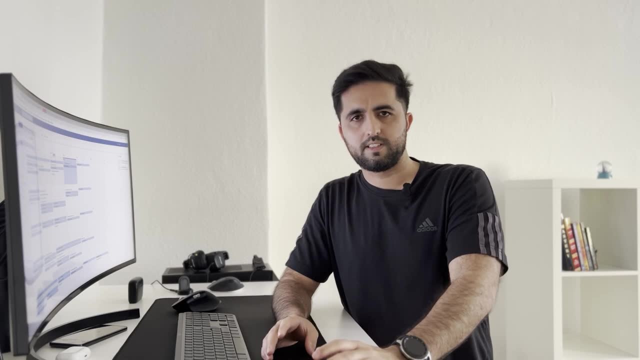 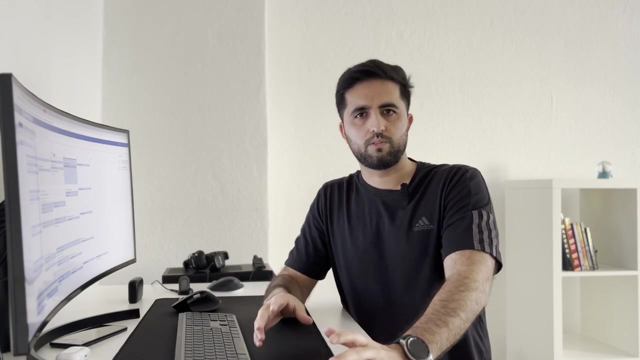 live environment or in the apps that people actually use. it can cause a lot of problems, and once these bugs make their way into the live product, fixing them actually costs way more than to have them fixed early on in the process. So companies are now integrating QA as part of the 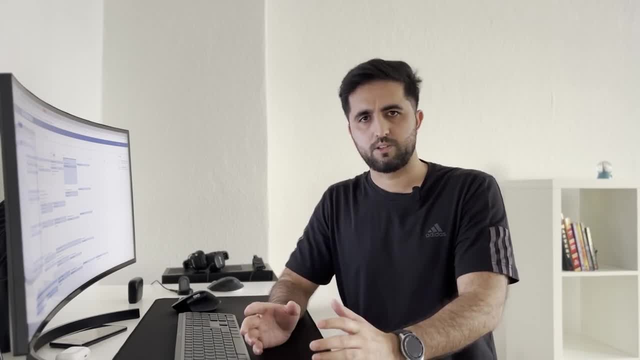 development team more and more and they're heavily investing in QA engineers and they are opening up a lot of roles in QA development. So they are now integrating QA as part of the development team more and more and they're heavily investing in QA engineers and they are opening up a lot of roles. 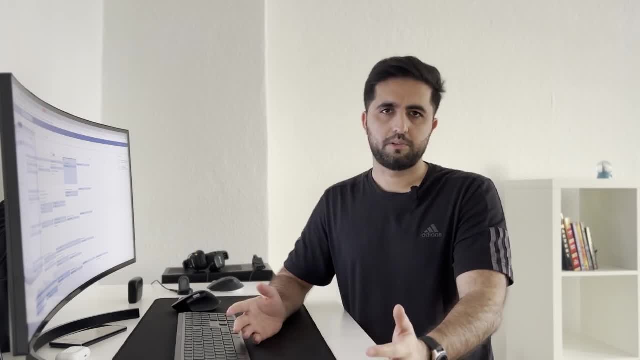 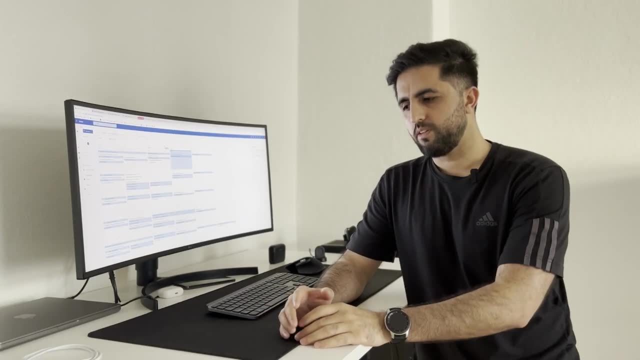 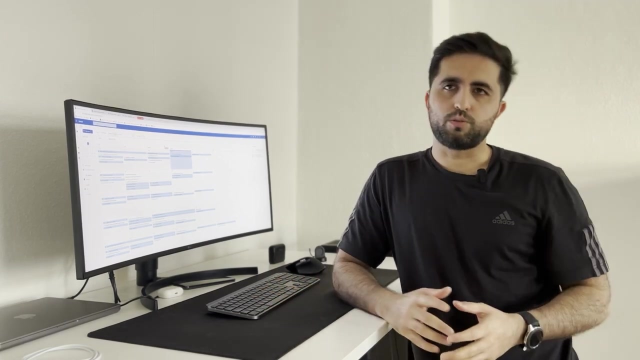 in QA. So now is a good time to basically look for a job in QA to start your career. So let's now talk about how I got into QA and landed my first QA role. I just want to start by saying that I do have a degree in computer science, which did help me get my first role as a QA engineer. 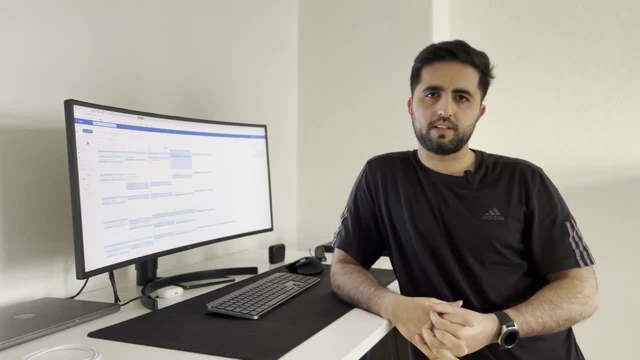 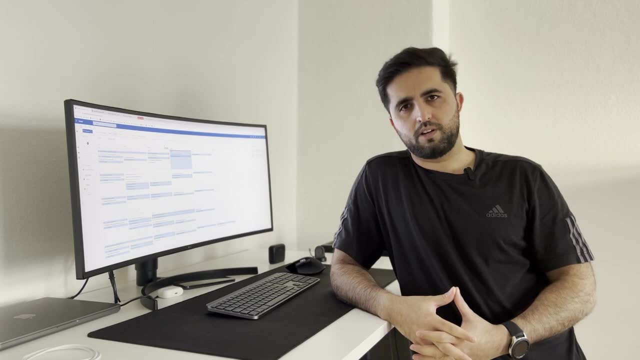 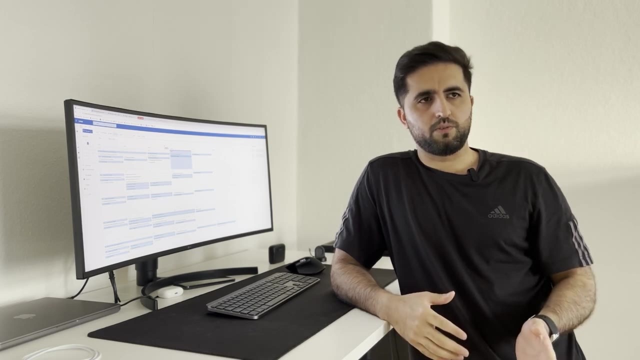 which was a part-time role, So I knew the basics of software development already and you know some programming languages like Java, some JavaScript, a bit of C sharp and basically a bit of everything. So it was a lot easier for me to get my first role. So I got my first QA job in 2017.. 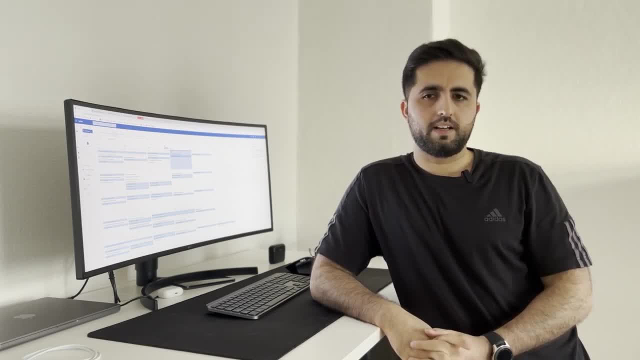 This was when I was studying in university and I was just looking for work because I need money and I wasn't super picky with jobs. basically, I was gonna take any job at that point, but I got called into an interview for this role as a QA engineer. I didn't know what QA was. 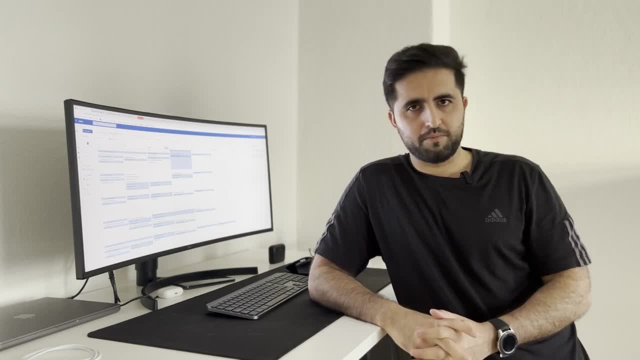 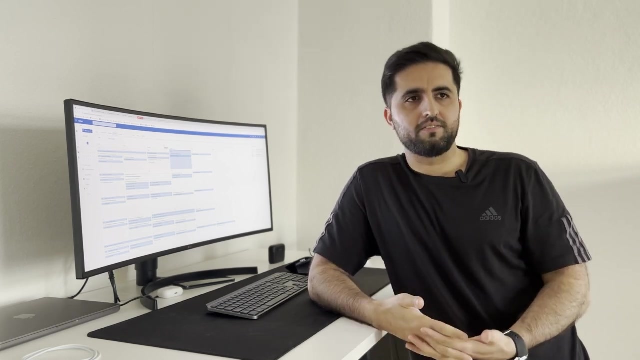 at the time. but I went in because the job description mentioned some of the technologies that I worked with, like programming, like with Java, and then it mentioned something about QA, which I didn't know. so but I went anyways. They interviewed me and they gave me the job. 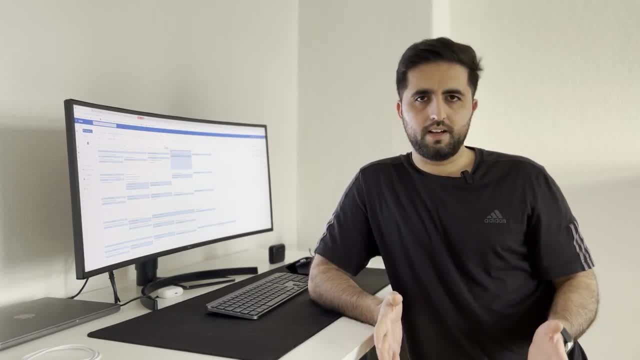 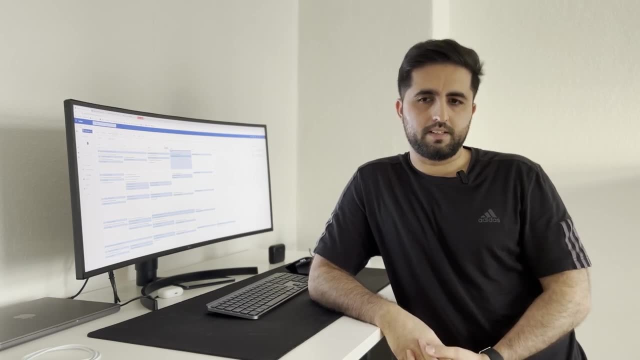 It was a part-time role and at this job I basically learned a lot about test and use my programming skills to kind of learn about automation, and I was doing a lot of manual testing as well. so the company that I was working for they had mobile apps, TV apps and also a web application as well, so they had a wide 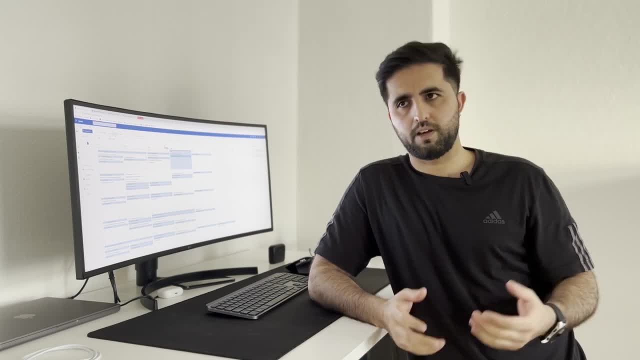 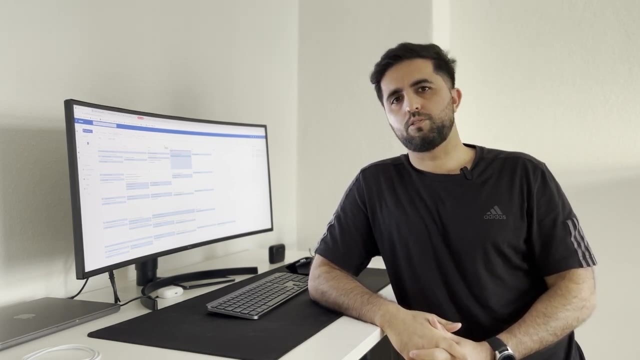 range of different applications on different platforms. so that was a good starting point for me, because I was learning to test on many different devices and many on many different platforms. so it was a good first experience. I worked there for about a year and then I decided to move to a 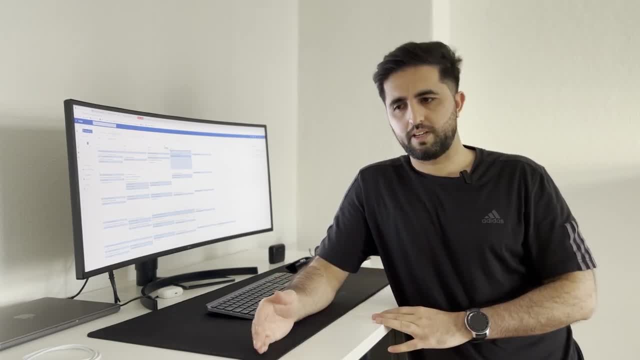 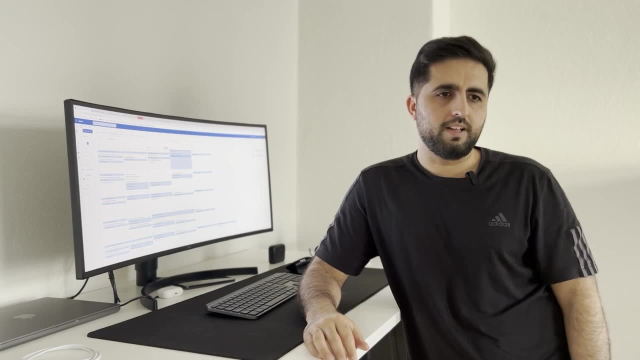 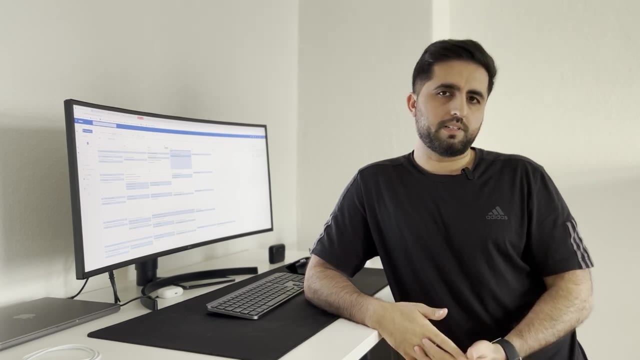 different company because the work that I was doing there was getting quite repetitive and I will, my learning kind of stopped at that point, so I wanted to try something different, so I got a job in a new company. so after working in the next company for about a year, they offered me a full-time role, which I 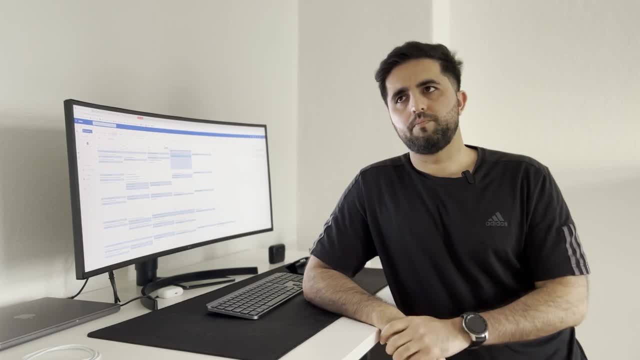 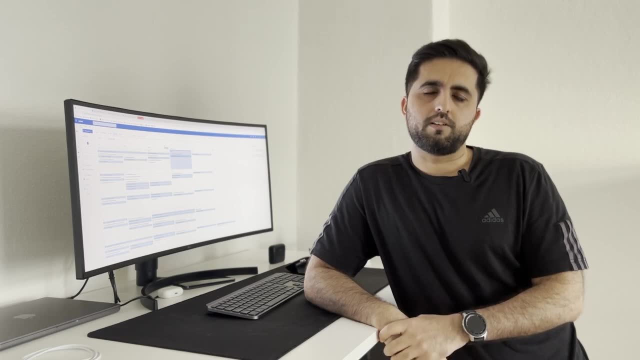 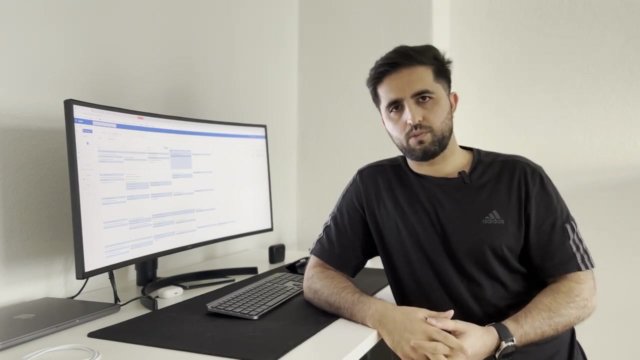 accepted and then I was doing automation for them and, yeah, also a manual testing. but at this point I had developed quite a lot of skills relating to QA: things like making test plans, organizing test runs, creating new test cases and deciding what to automate, what not to automate. 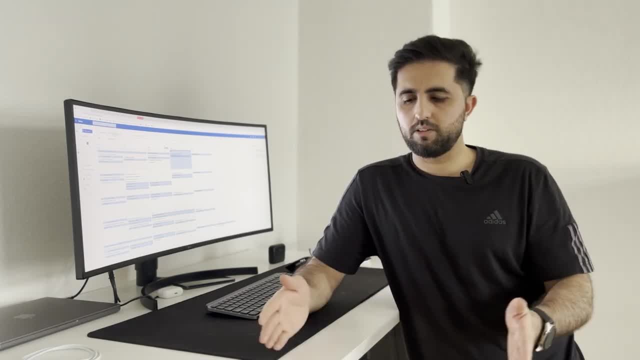 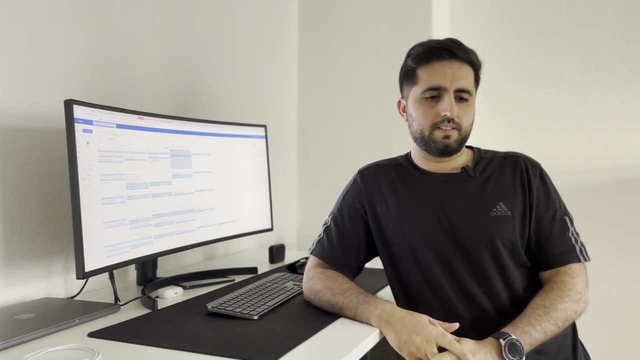 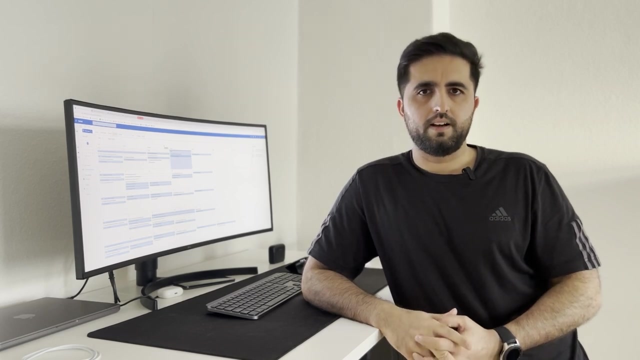 and a bunch of other stuff. I learned all the basic QA processes in this company. right now, I'm working for a company called Deep Health. they basically have an AI based translator which works on Windows, Mac and iOS, Android, so it is AI based language translator. it's one of. 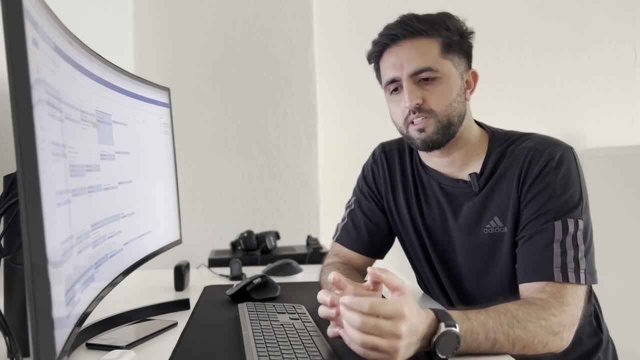 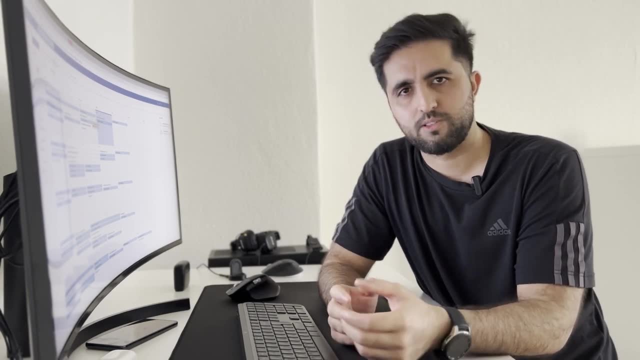 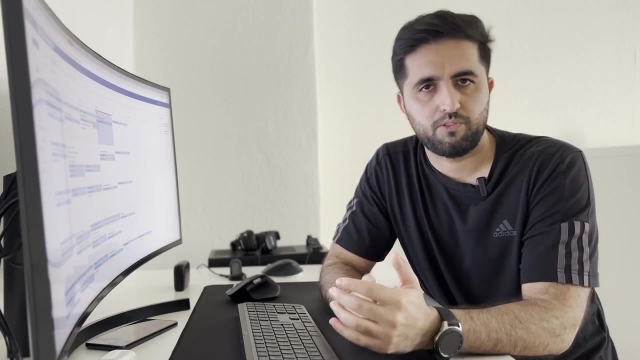 the best out there. I think the most fun aspect of my job is finding bugs. it's something that I enjoy the most just doing lots of regression testing, smoke testing, just to find and basically break things and make sure that I find the bugs before a user does right. 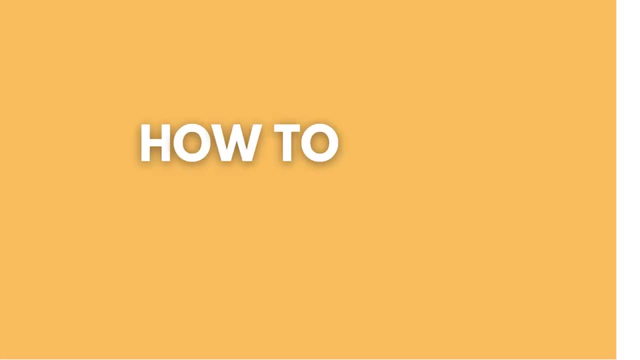 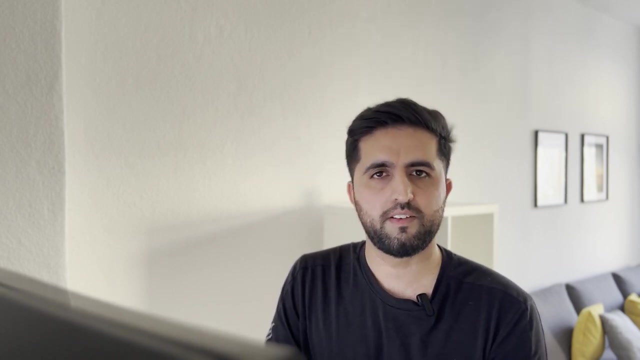 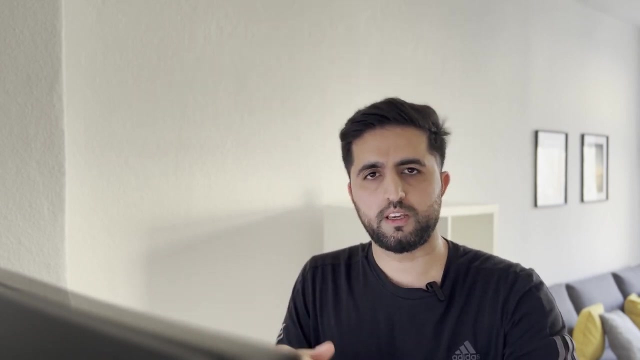 Yeah, so this is my QA journey, All right. so for people who are not from a IT background, who doesn't have a degree in computer science, you can still get into QA, because most of my QA colleagues in the past they didn't go to universities at all. 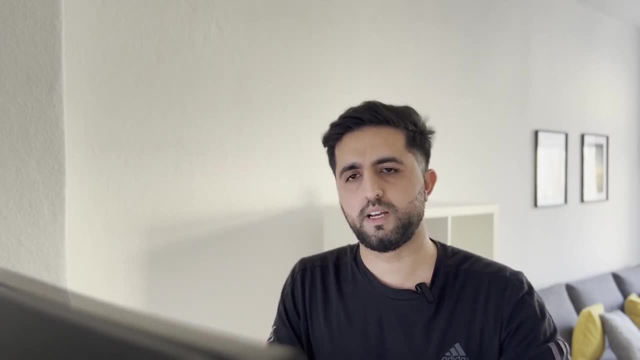 Only few of them did. They were the QA teammates that I had in the past. They basically did a course somewhere, maybe six months long intensive course on QA. Some of them did a IST QB certification and then started taking up part-time roles. 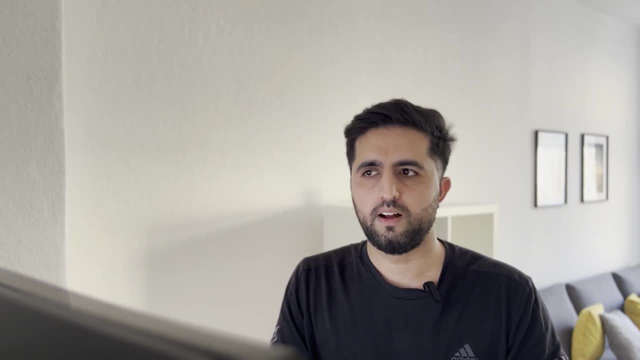 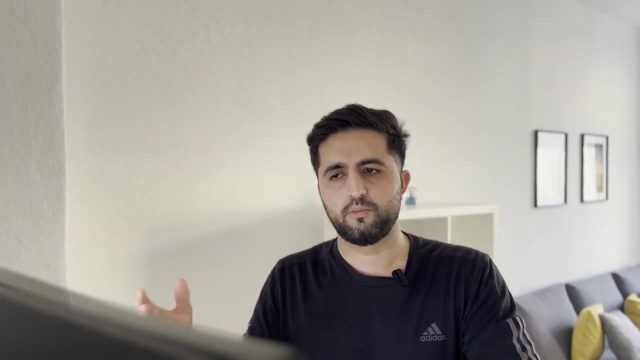 Some of them did internships in the beginning. I mean, the downside of that is that you won't get paid much in the beginning, but you can't just get a full-time role straight away if you do like a six-month long course on QA. 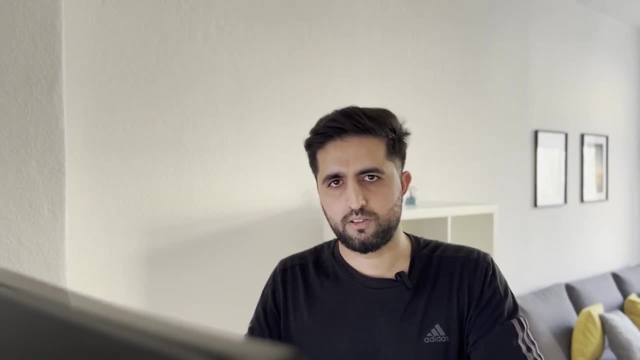 So maybe do two or three internships, which may be six months long each, So that way you can just gain some experience and also develop your skills and then start looking for full-time roles after that. So there's courses that you can do on Udemy as well. 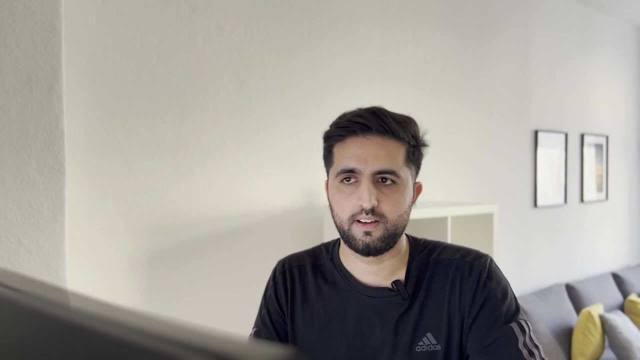 which you can do at your own pace. There are courses on YouTube as well, LinkedIn Learning as well. I'm gonna mention the links to some of those courses in the description down below, but I personally haven't taken them, but I'm gonna look at some of the ones. 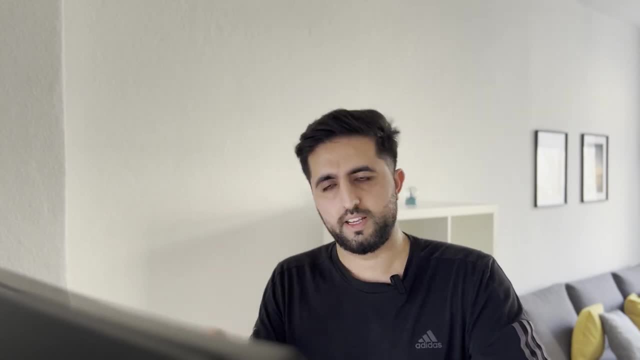 that have good content in them and then post the links down there. So if you have the basic understanding of QA processes, for example, then you can maybe start learning some programming languages, maybe Python. Python is a good start. It's easy to learn. 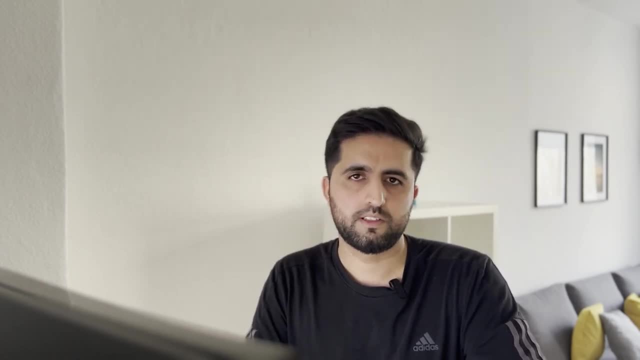 You can also start with JavaScript or JavaScript or Java, for example. These are widely used languages for test automation. Keep on working, keep on developing your skills and, yeah, you'll get there. It's gonna be difficult in the beginning. 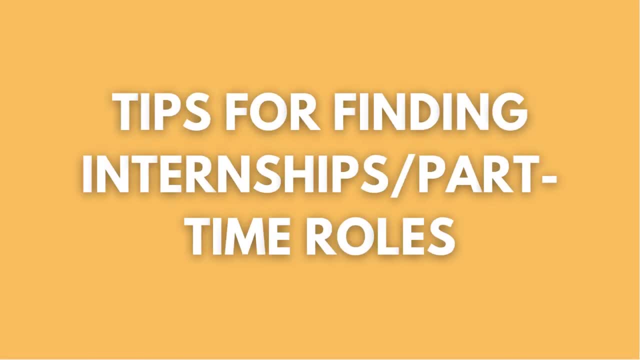 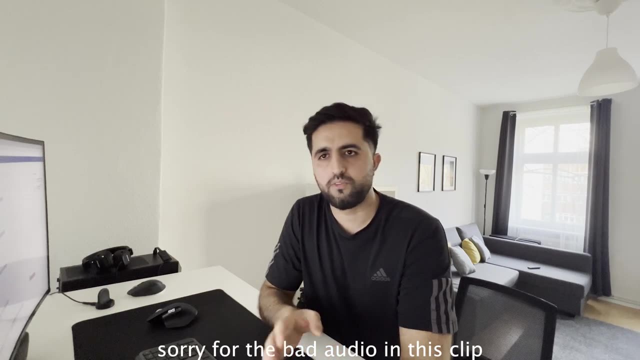 but it gets easier with time. So I have a tip for people who are looking for internships or part-time roles. in the beginning, What you can do is find any company that you like and write them an email that you can do an internship for.